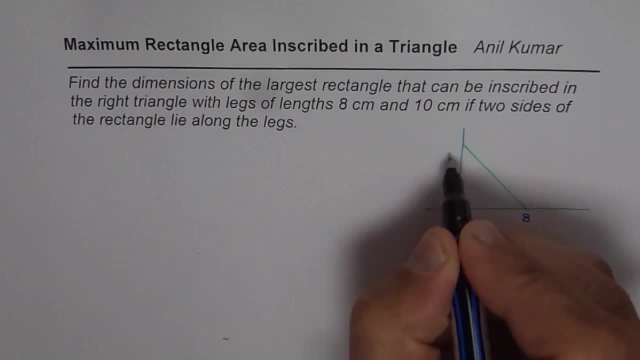 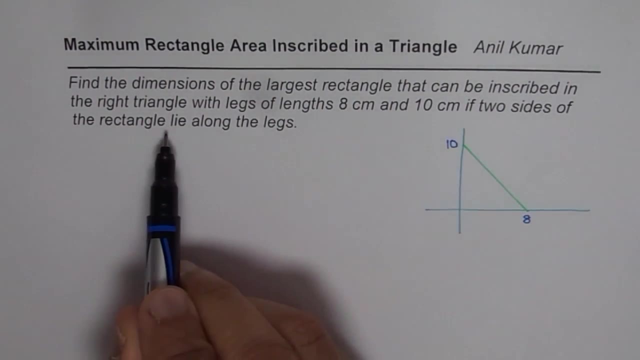 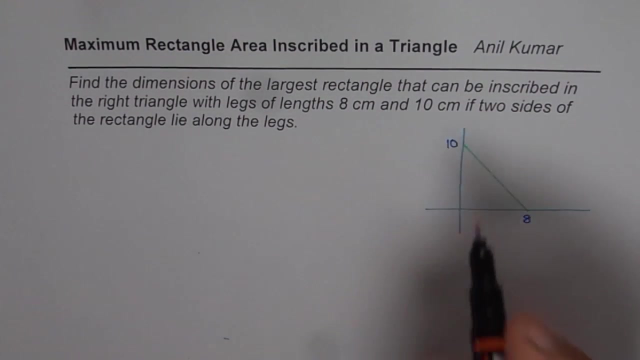 Let us say: this is 8 for us and that is 10 for us. So that is the triangle we have. Now we need to inscribe a rectangle with maximum area inside this particular right triangle. So that is right triangle. and, for convenience, what we have done is we have drawn it along x and y axis. 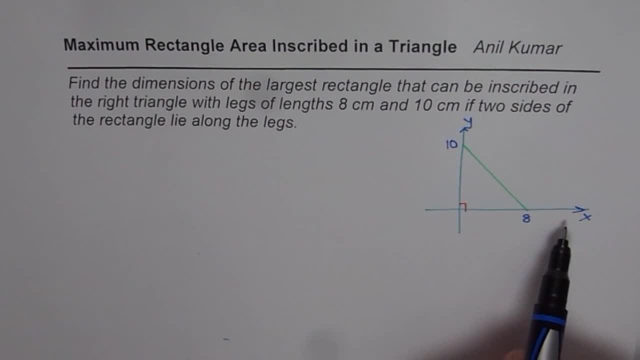 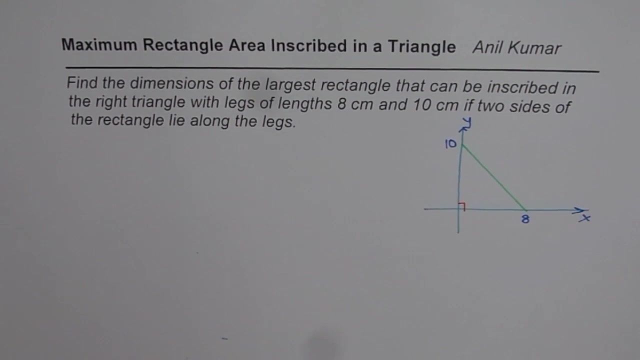 It always helps because when you are working in a Cartesian plane you can actually get the equation and then solve things better. So the idea here is somehow relate the variables. So we are saying that the two variables are x and y for our rectangle, And where is the rectangle? The rectangle is inside the triangle. 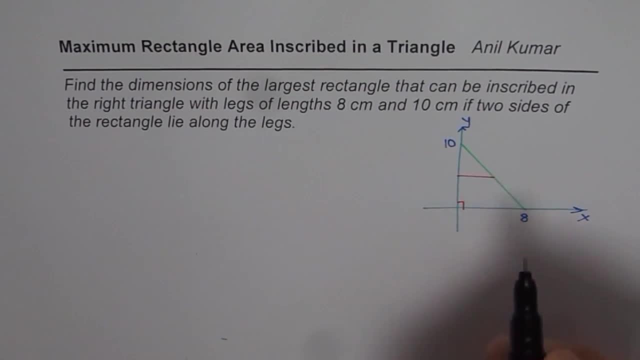 So let us make one. So let us say: this is the rectangle for us. Now we don't know what the dimensions of this rectangle are to maximize its area, But let us think about it in a general way. So let us take this corner. 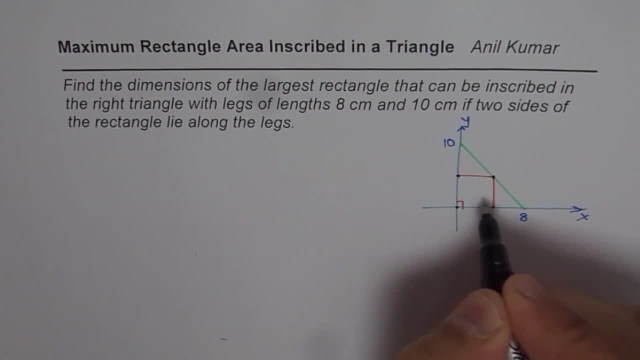 So these corners of the rectangle will actually be as shown. So always all the four should be on the sides of the triangle so that it can be inscribed inside it. Now let us consider a point on this hypotenuse of the triangle. So let us say in general: 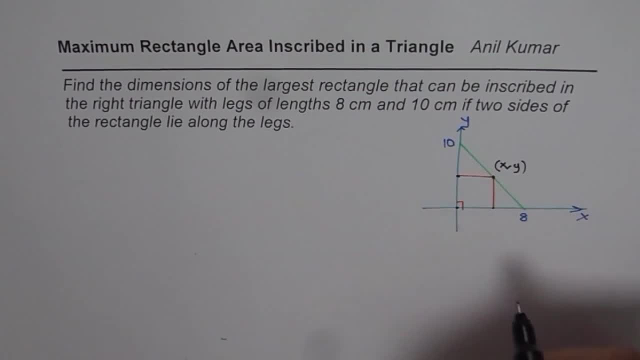 this point is xy. So any value of xy. What does that mean? It really means that length of this rectangle is x, that is to say, this distance from here to there is x and y is the height of this rectangle. So from here, 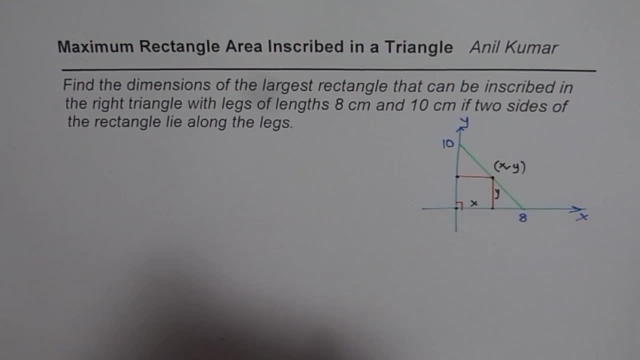 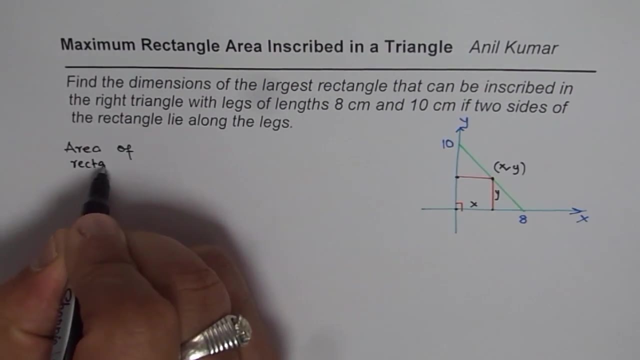 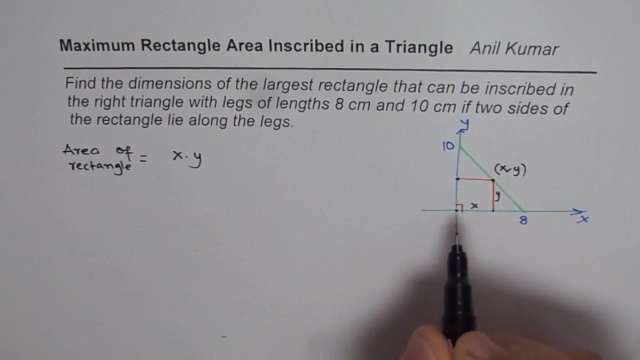 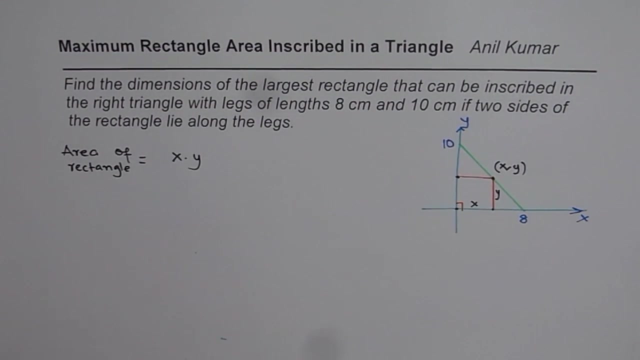 you can get one relation about area of the rectangle. So what is the area of the rectangle? We can write down: area of rectangle is equal to x times y. Now the objective is to maximize this particular area. So whenever you have an equation, you need to somehow relate the two. 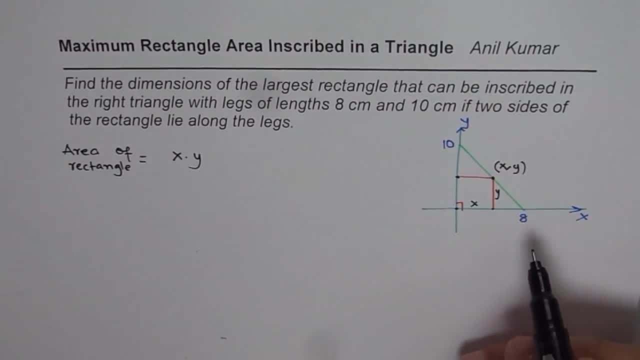 variables which you have taken Two or more, In this case just two. Now, here you will see one way to relate them is similar triangles. So one way is to use similar triangles to relate them other ways. we will get to that. also Other ways to find the equation of a line. 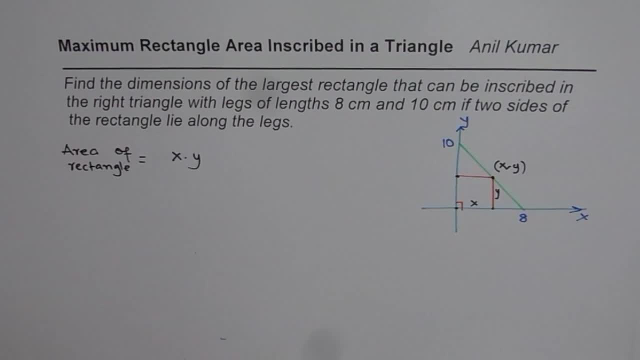 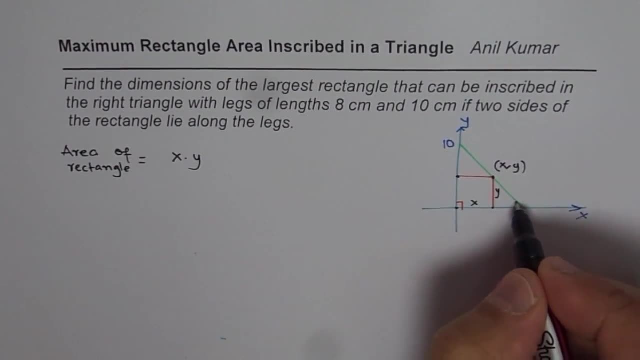 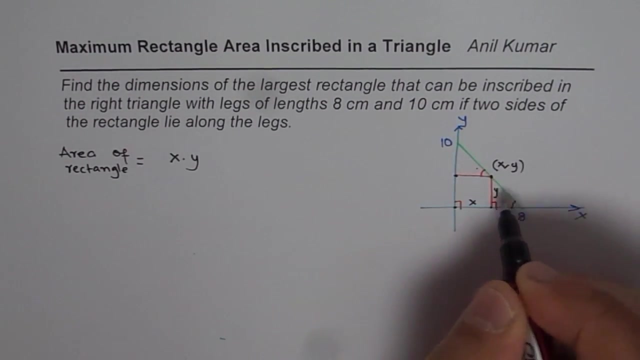 which relates the two. So we have two different approaches in such questions. We could do similar triangles. Similar triangles means that you know this angle is equal to this angle and then we are working on 90 degrees. I mean we can take small triangle and the big triangle. 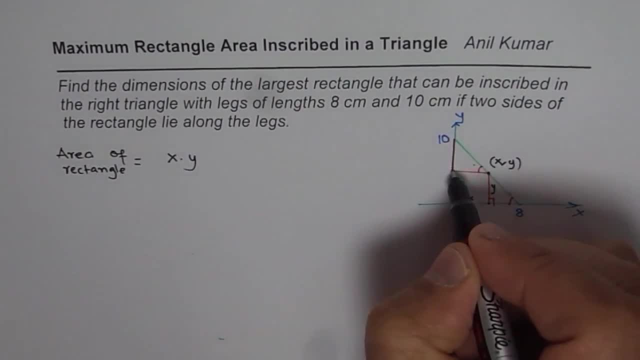 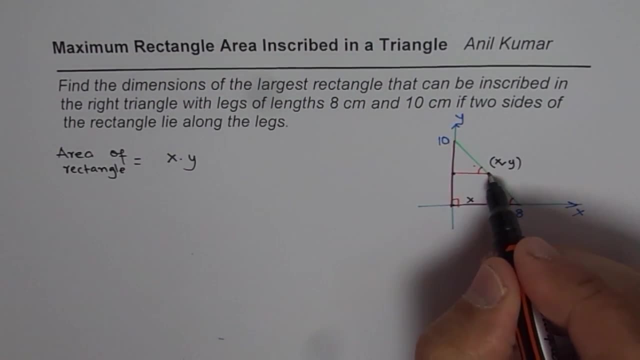 as such. So let us consider the big triangle, which is the triangle given to us, whose sides are 8 and 10, and the small triangle, which is this one for us. Now we will do one method using similar triangles. Now, in this case, from similar triangles, you can relate. 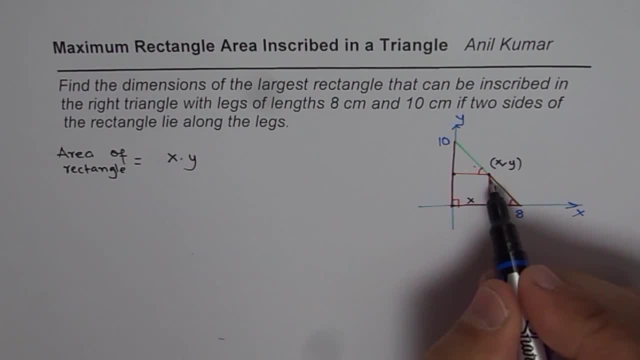 x and y. We need to find what y is in terms of x. So in a small triangle, y over this side is how much? Since the total base is 8, that should be 8 minus x. So we are talking about this side, So that side. 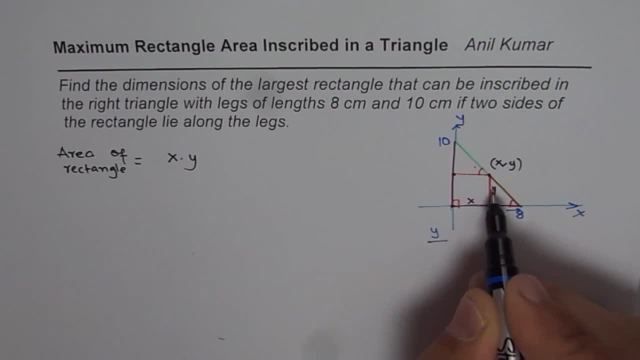 is 8 minus x. So we could write this as: y over 8 minus x is equal to: for the big triangle it is 10 over 8.. So that relates the two. So that is y equals to 10 over 8 times 8 minus x. 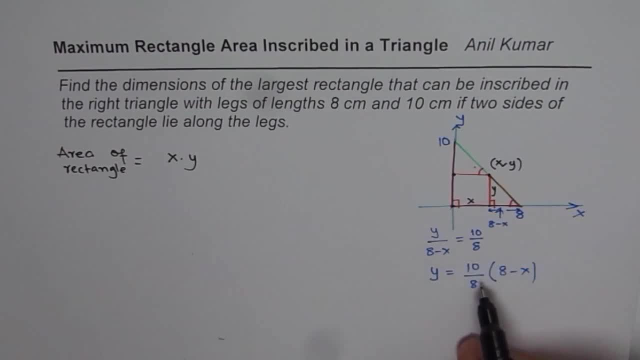 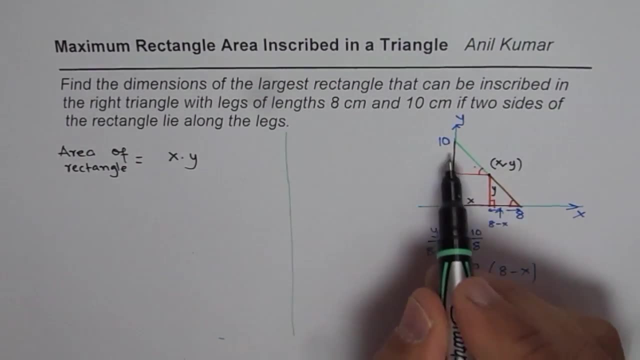 So that is the relation you get from similar triangles. The other approach could have been to use equation of lines. Let me show you that also. If you have this equation, let us use equation of line. The y intercept is 10 and the slope is minus. 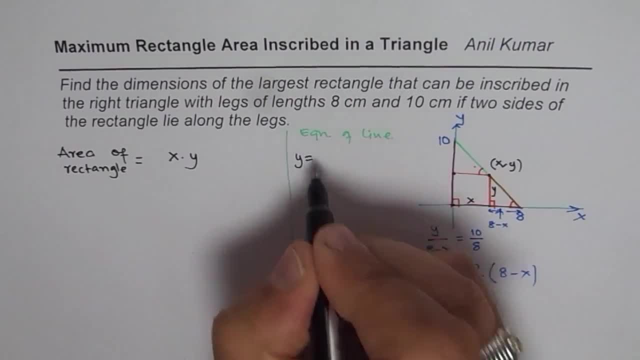 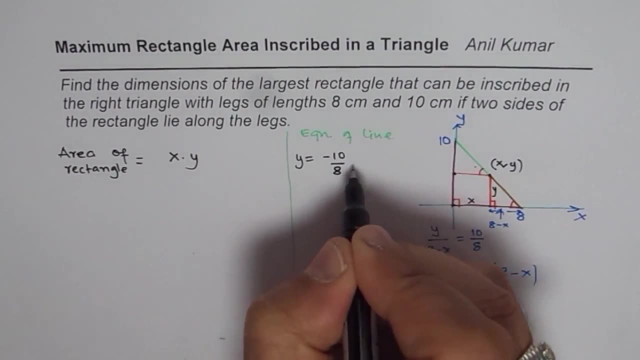 10 over 8.. So we can write equation of line as y equals to what is the slope. You can go down 10 units and write 8.. So it is minus 10 over 8 x and the y intercept is 10 plus 8 plus 10.. 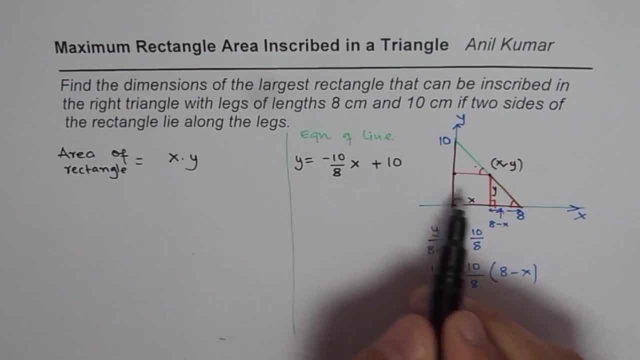 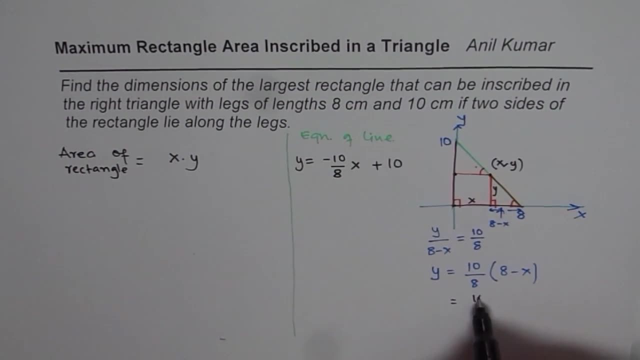 So you could use equation of line also to get this relation. You get the idea right. So it is exactly the same relation. So if you expand this, what do you get? You get 10 minus 10 over 8 x, right? I am purposely not? 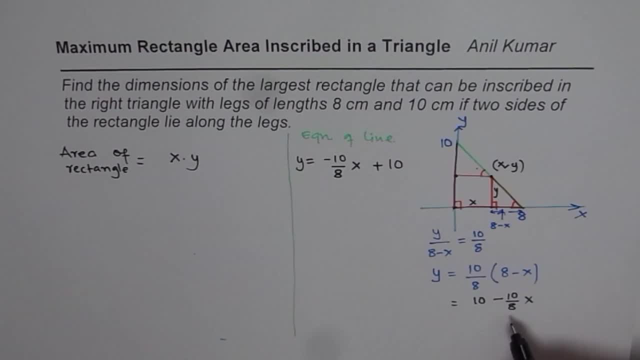 simplifying this to show you some of the relations which will develop as we saw. So these are two different ways of relating y with x. One we used similar triangles- Very helpful similar triangles- And the other equation of line. At times the equation of line can be given to you. 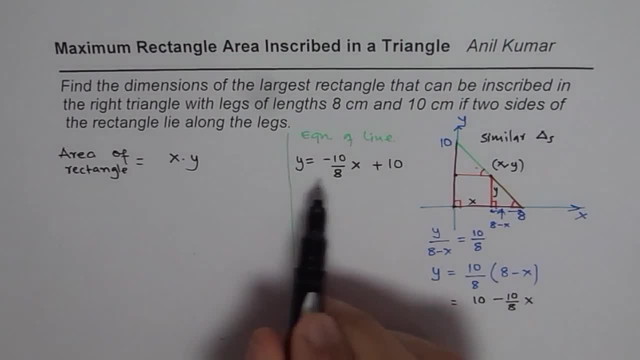 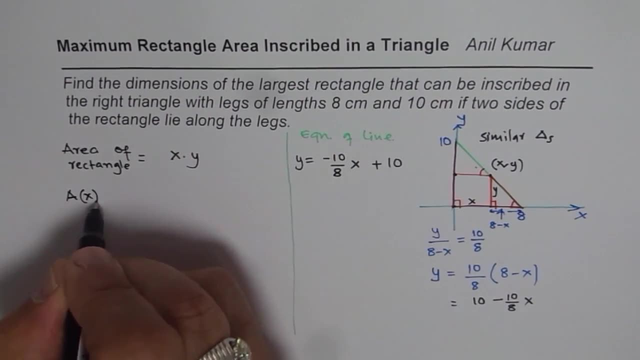 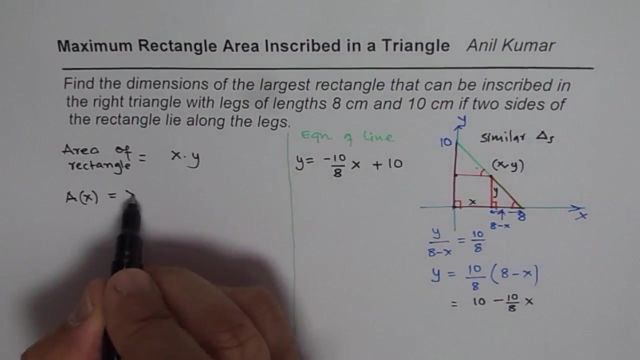 So the idea is to relate the two variables, which we have done. Now we can say area in terms of one variable, x. So we are defining a function. Area is function of x, now where x is along the base of this triangle And we can write y. 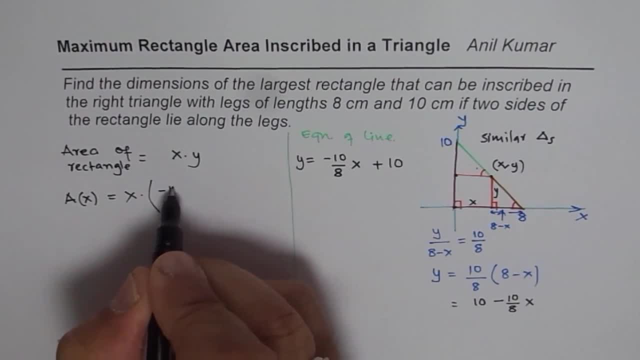 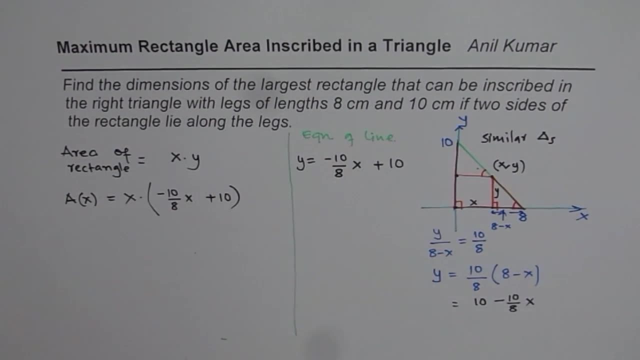 as we defined here as minus 10 over 8, x plus 10, right. So we get the area in terms of x right Now. to maximize this area, we need to find the critical points and also we can check what is the area at the extreme. 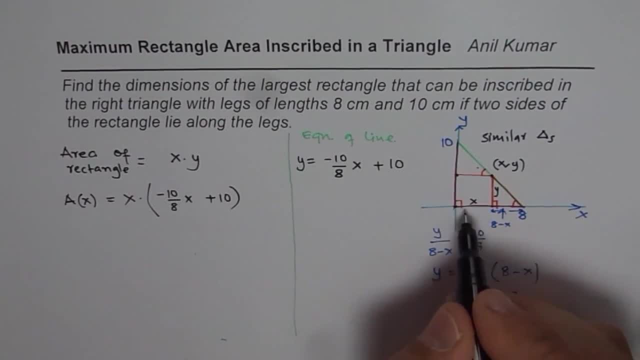 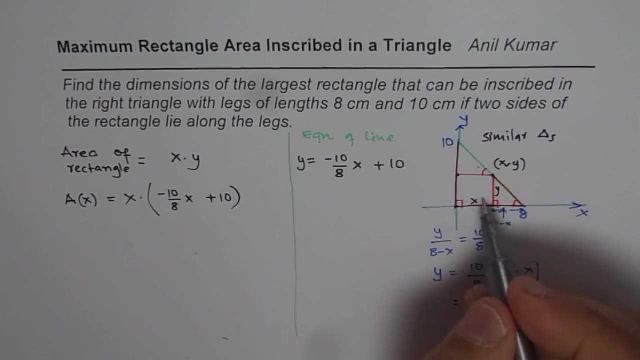 values of x. As you can see from here x, this triangle could be a very wide triangle. For example, the x value, it could be kind of approaching like this big right. So x could approach 8.. Do you see that? 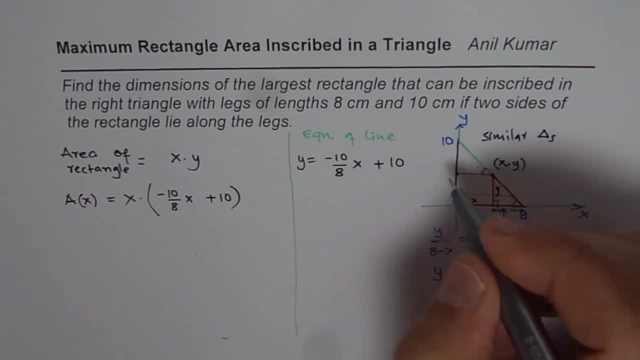 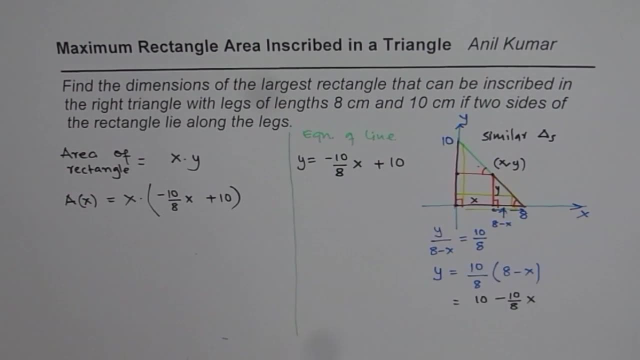 So that's the maximum value x could have. Or it could be a very thin but tall triangle like this, where x is approaching 0.. You get the point. So what we can do here is we can say what are the boundary conditions for x? We say x. 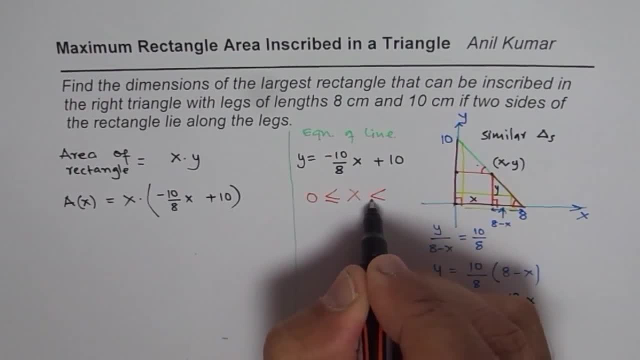 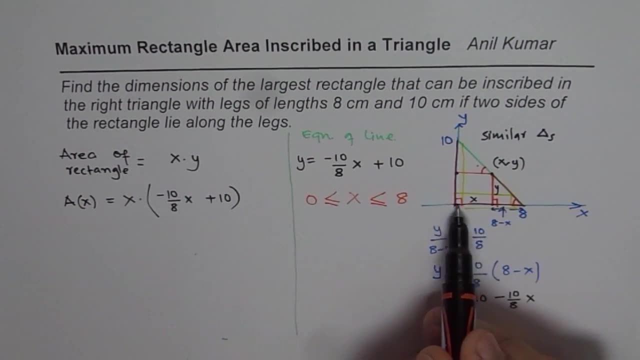 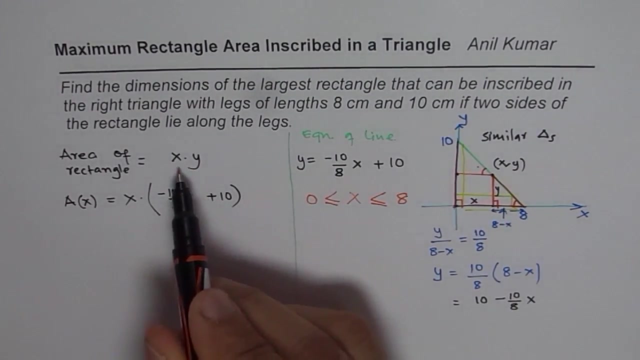 could be greater than equal to 0 or could be less than equal to 8.. Now, as you can see, in both these triangles, as x approaches the extreme value of 0 or 8, its area becomes 0,. right, Because if x, 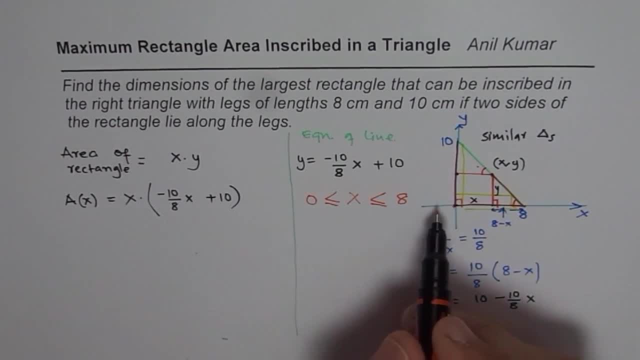 is approaching 0, 0 times, anything will be 0. If x approaches 8, then y will be 0, right? So in both these cases, what you find here is that the area for the triangle for x value of 0 is 0. 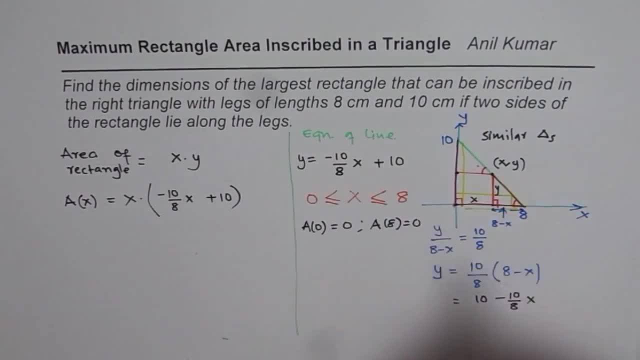 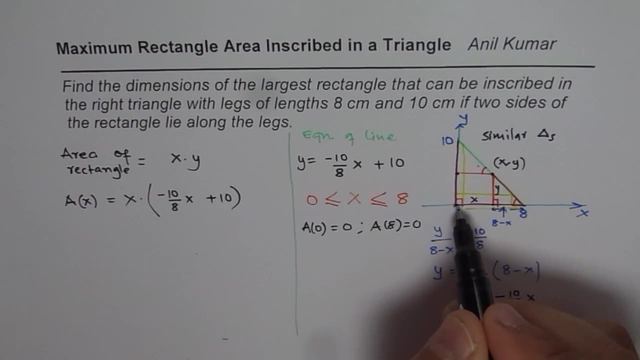 And for 8 is also 0. Now that gives you an idea that somewhere in between it is maximum. Do you see that? And as most of you must have guessed it, it is maximum when x is just half of it. right Now, that could be. 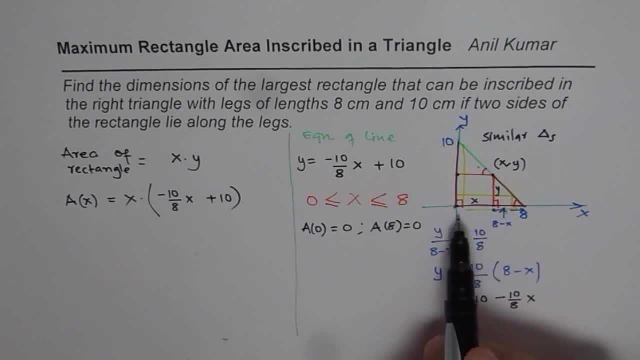 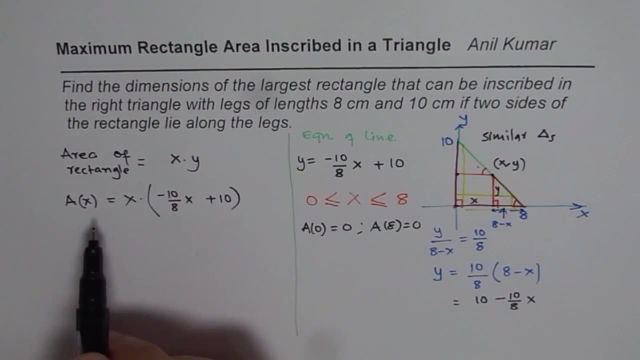 a question at times to show that for half of the width it is maximum area, right, So there are different options. But anyway, you get an idea, Let's try to prove it, or rather find it out. So we have from boundary condition. 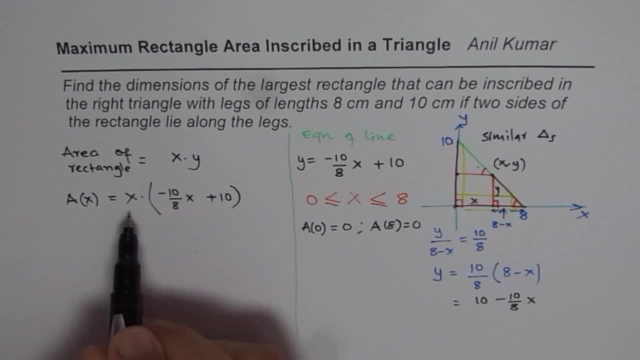 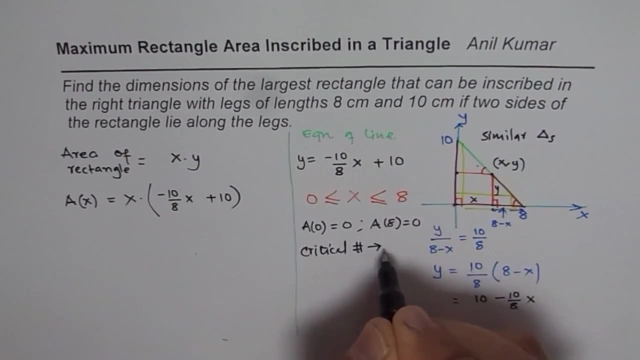 a very clear value that whatever critical point gives us, it is a maximum. So we know at critical point we have a maximum, Is that okay? So at a critical number or point we are looking for maximum area, correct? So that is all the. 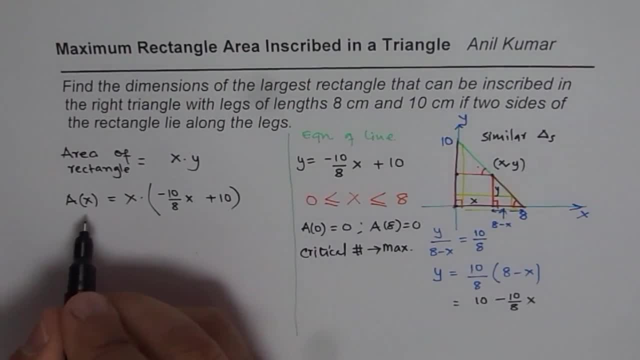 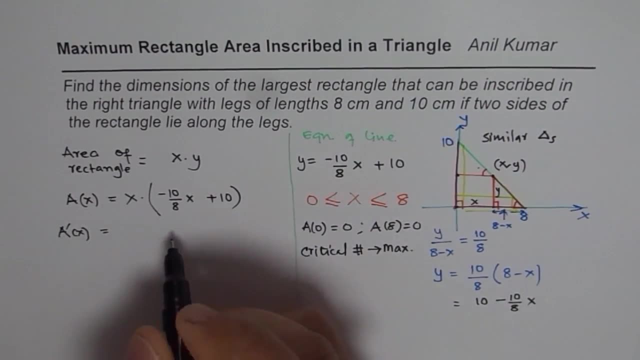 thinking, which you have to do while you solve. Okay, Now let's continue with solution. So we'll find the derivative of this function with respect to x, right, So you could do one thing when you are finding derivative Before even finding. let us expand. 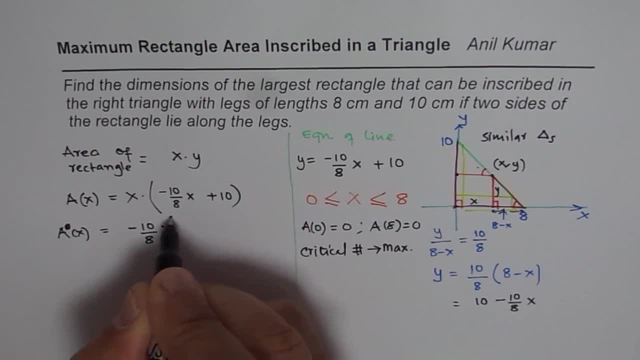 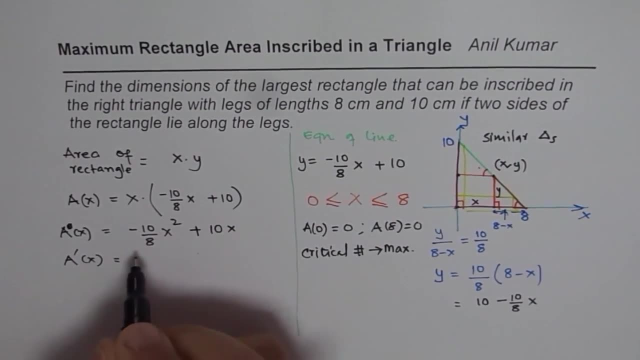 this. It becomes simpler. So we'll expand it right. So we'll get plus 10x, correct. Now we'll find the derivative right. So the derivative for this is minus 2 times 10.. So I'm writing: okay, 20. 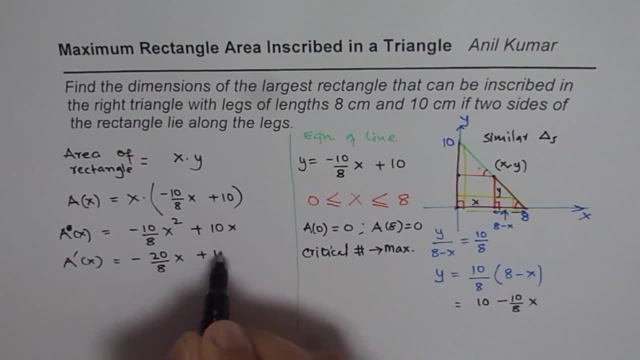 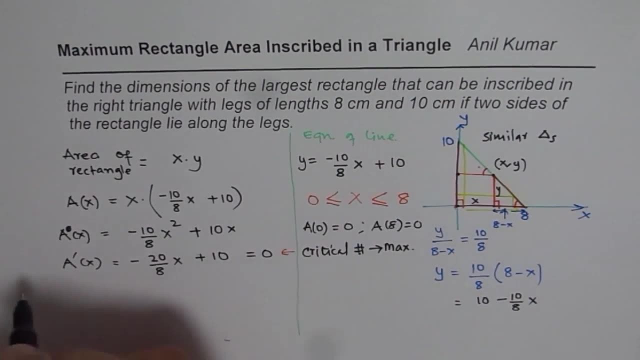 over 8x, and here we get plus 10, right Now we need to equate this to 0 for our critical point. right, Or critical number. right, As you see, critical point means that you have to find y. 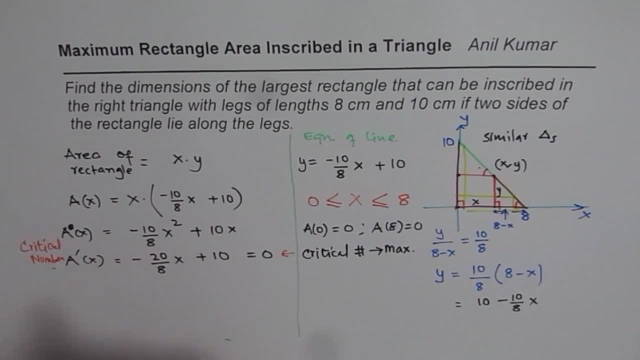 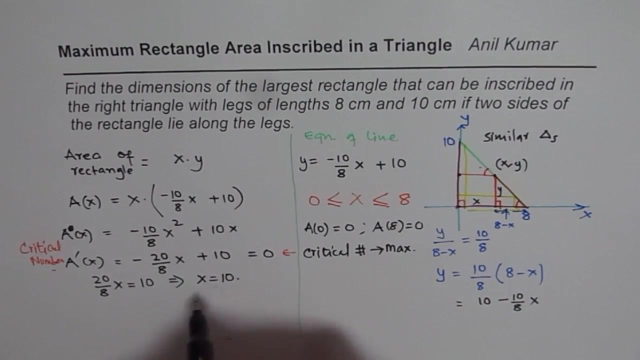 also. So we say number, since we are only finding x value. Okay, Now this will be 0. That is to say that 20 over 8x equals to 10. And that gives you the value of x as 10 times. 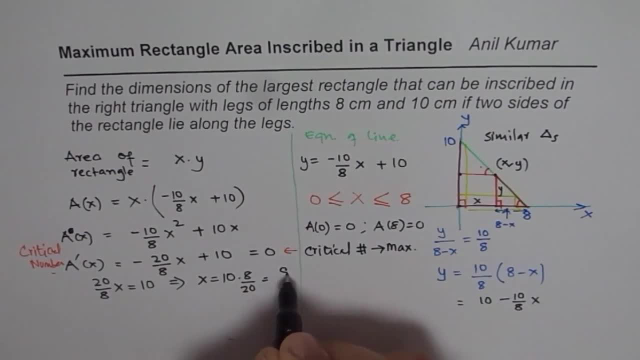 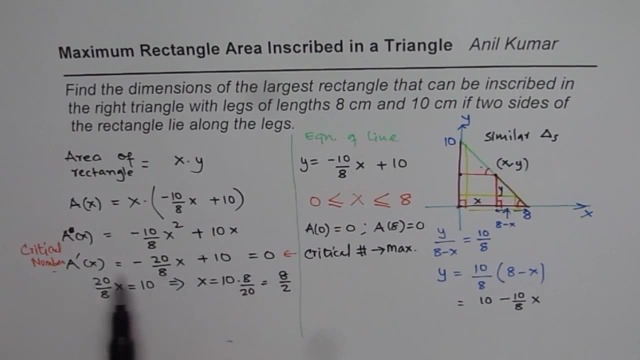 8 over 20, or it is equals to half of 8.. Do you see that, Whatever, the base was half of that. So that is the value of x, for which we get a critical number, and we know that will result into maximum area. Well, 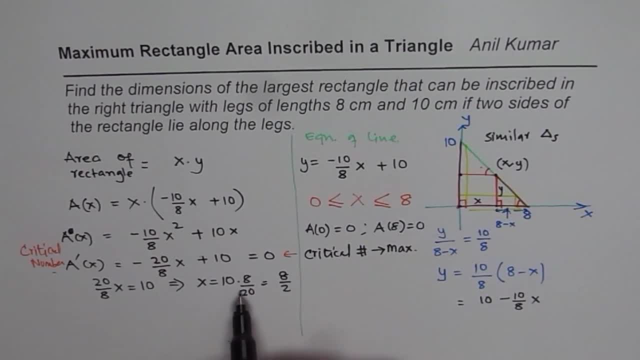 you can find the dimensions If you substitute x as half of 8 in your equation. you can find what y is right. So for getting the dimensions, let us find y value also. So y should be equals to minus 10 over 8x. 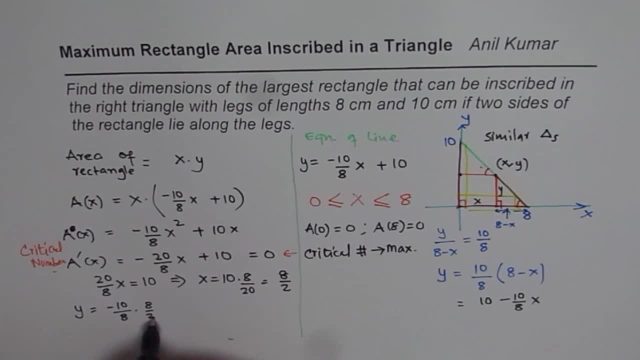 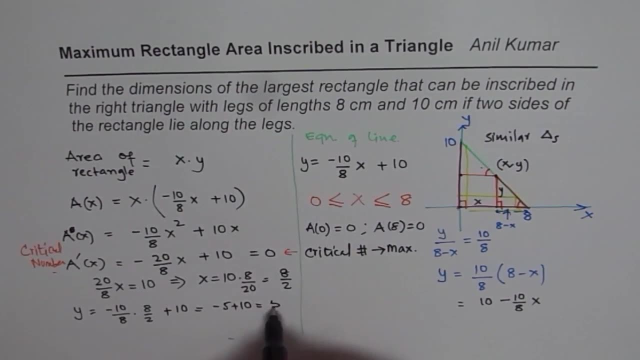 which is half of 8, right? So I'm writing 8 over 2 plus 10.. And that is half of this, So minus 5 plus 10, which is indeed 5.. So, as expected, our dimensions are half of 8, which is. 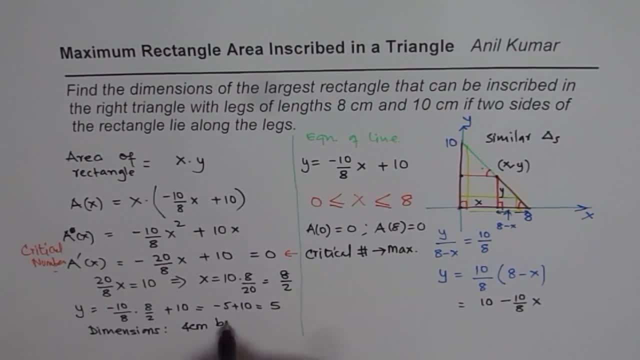 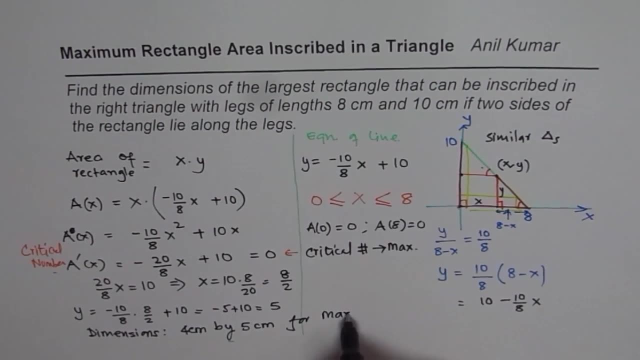 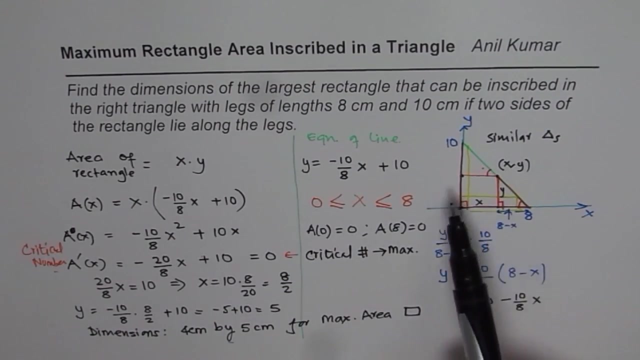 4 cm by half of 10, which is 5 cm for maximum area right of rectangle inscribed in this particular quadrant. So at times I could ask this question like: if there is a line in coordinate 1, then what is the area of maximum? 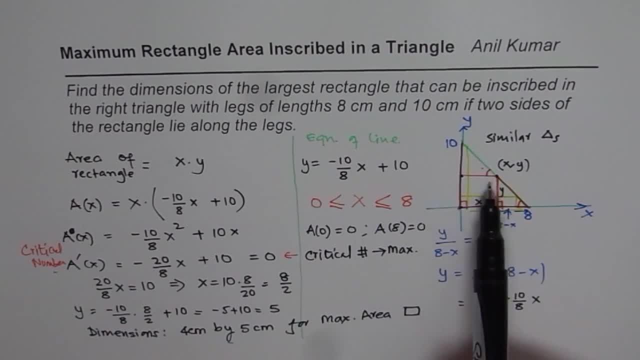 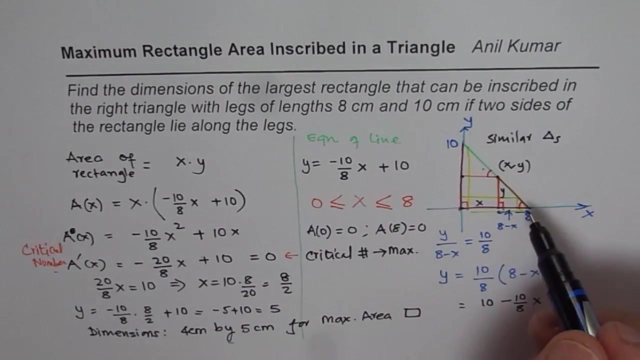 inscribed rectangle which it makes with one corner on the line and the sides along the x and y axis. So these are different ways in which we can ask this question. as an exercise, What you can do is you can generalize this question, That is to say, now you can take 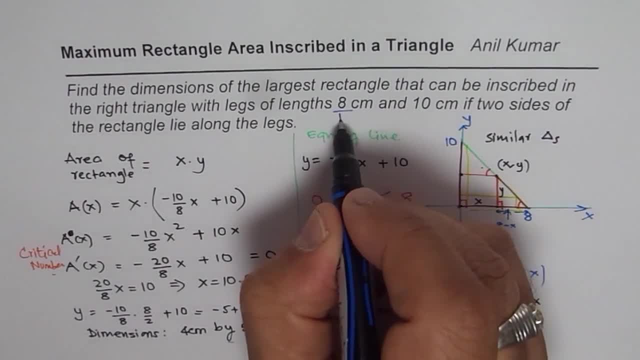 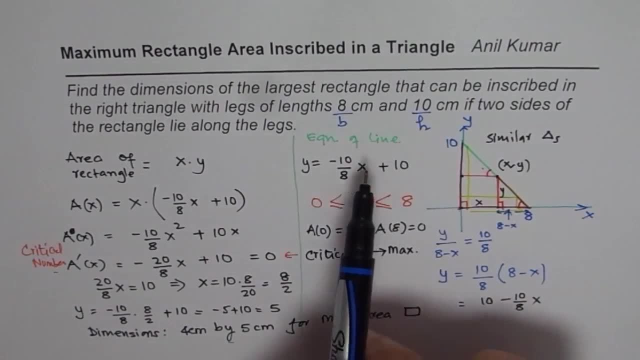 any value. So if you take base with b and height as 10, right, In that case, if you replace these values with b and h, if b is the base of the right triangle and h is the height of the right triangle, in that case, 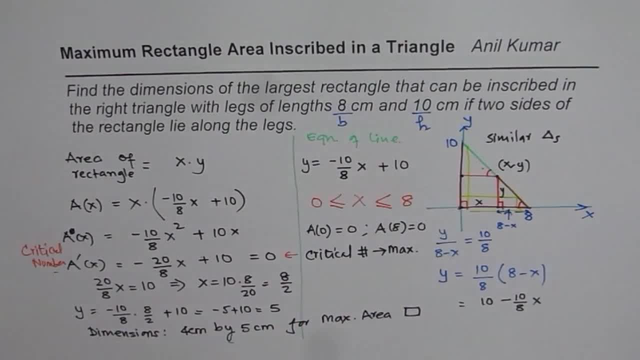 find the dimensions of largest rectangle. So that question you can also solve with the same method. and you expect the answer to be half of base and half of height. So that gives you the answer for the given question, right, If you kind of generalize it. 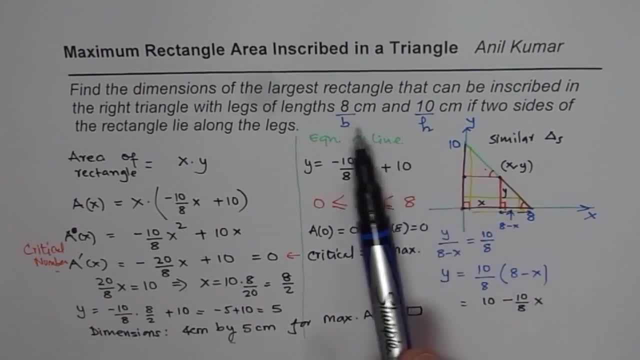 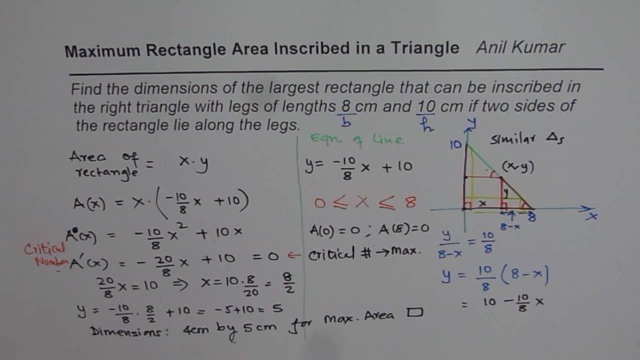 you will find that in any triangle it works right. So that is kind of interesting and important to explore. So I like you to explore all these combinations and then move on to similar questions. Thank you and all the best.